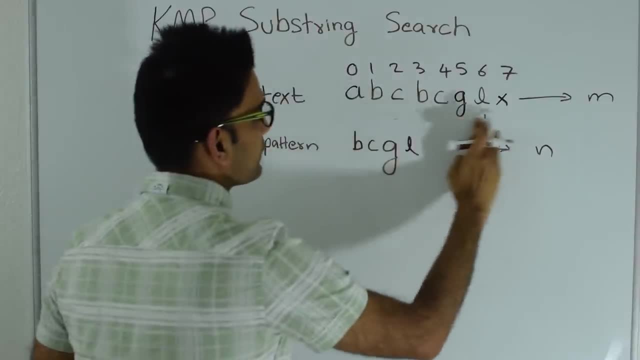 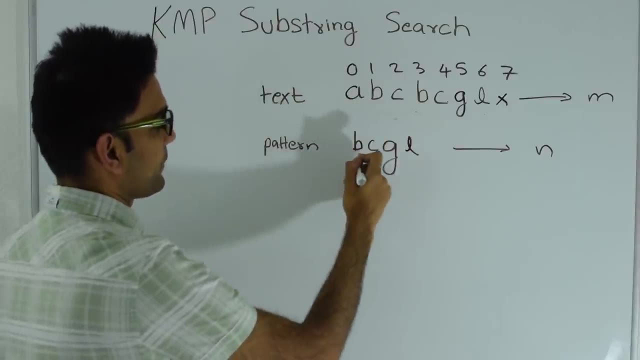 usual algorithm to find the substring search. What we usually do is we start from this, from the 0th index of the text and 0th index of pattern, and we compare B with A. Since they are not a match, we go to the next index of text. 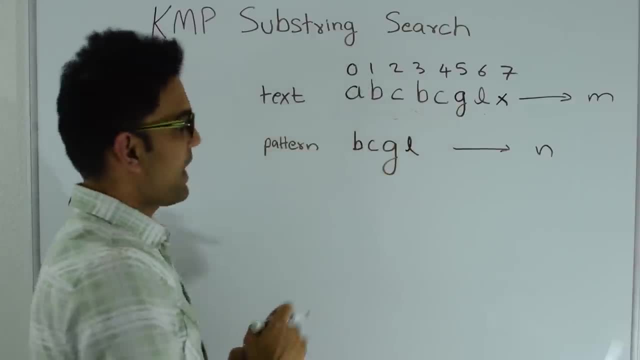 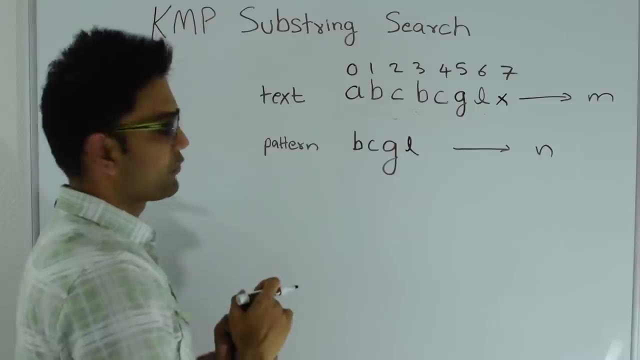 which is B. So we compare B with B. Since it's a match, we compare C with C- Again it's a match. so we compare B with G. At this point it it's not a match. So what we do is we start from the next of the start point. 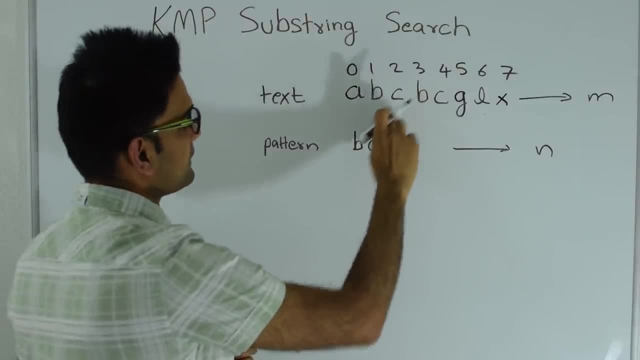 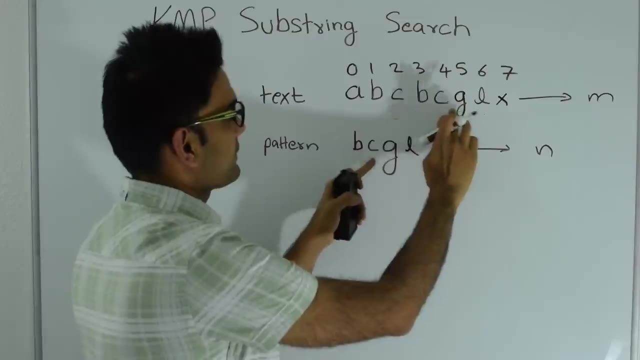 So then we start from C and then we compare C with B. Again it's not a match. So again we start from the next point, then we compare B with B. So this is a match. and then C is a match, G is a match and L is a match. So in this case we 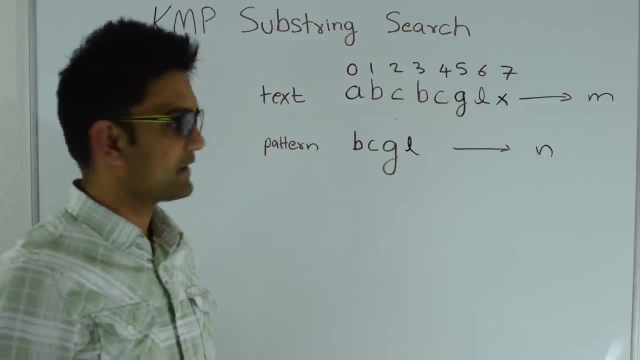 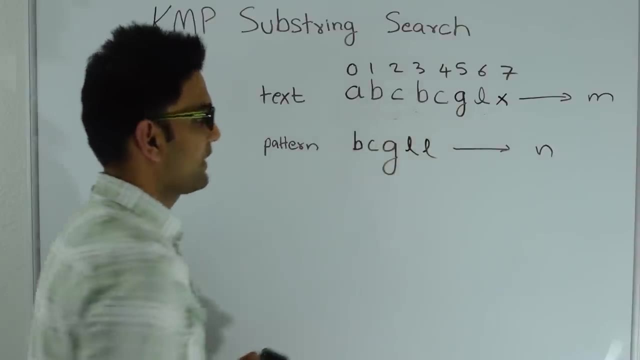 would return 3, which is the index of the point at which text exists, and if our pattern was something like BCGLL, in that case this pattern would not be found in the text and we would return an exception or minus one or something like that. 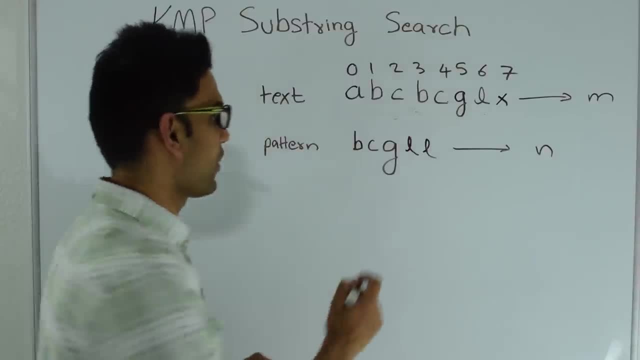 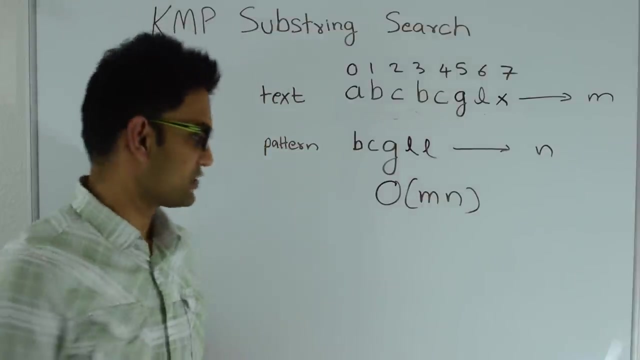 So how much time would this algorithm take? In the worst case this algorithm would take O time, where M is the length of the text and N is the length of the pattern. So this is where KMP search comes into the picture. The KMP search can do the substring search in: 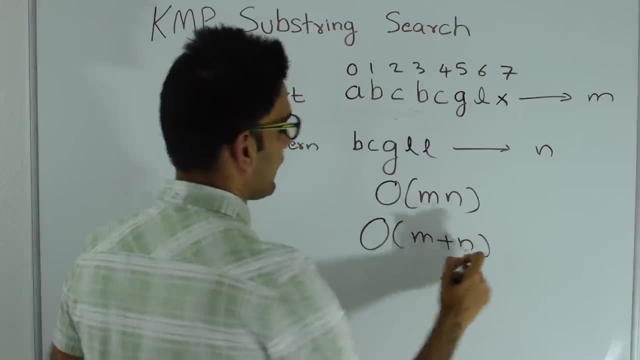 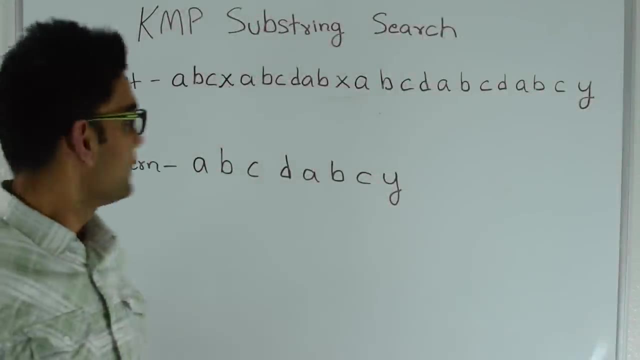 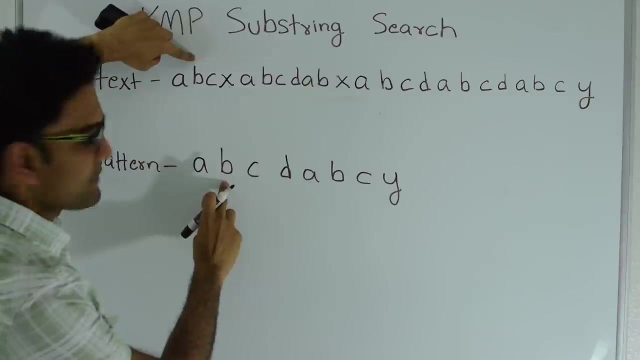 O M plus N time. and let's see how KMP search works. Let's understand KMP algorithm using this text and this pattern. So we start from here: A and A is a match, B and B is a match, C and C is a match, D and X is not a. 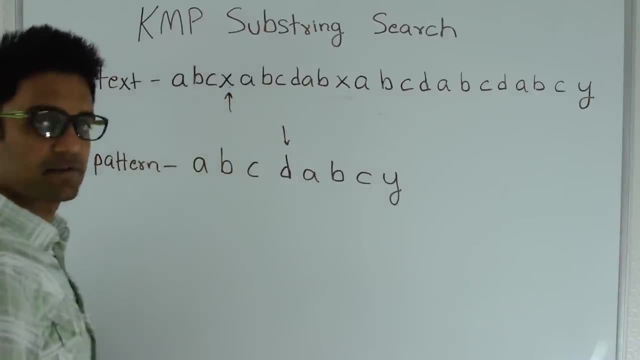 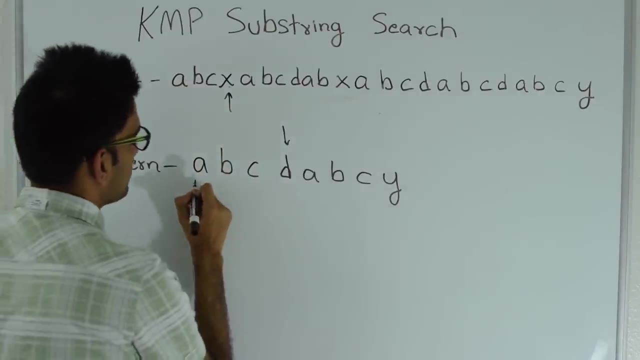 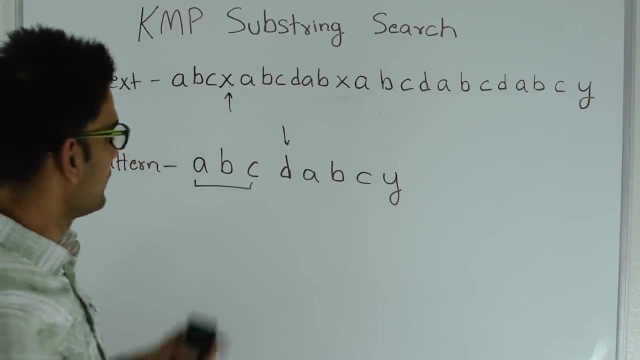 match. So this is the point: we find no match. So our aim is to not go backwards in this text. So what we are checking is: right before D in this substring, is that a suffix, which is also a prefix of this substring, Since all the 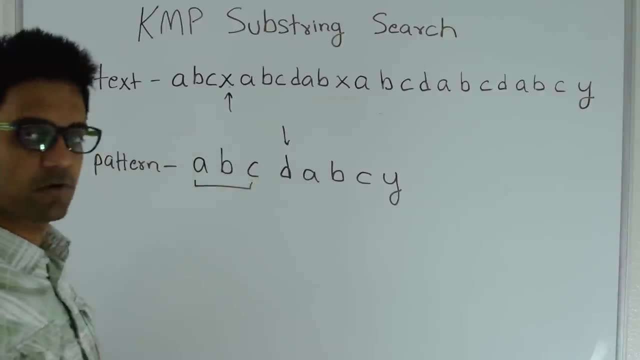 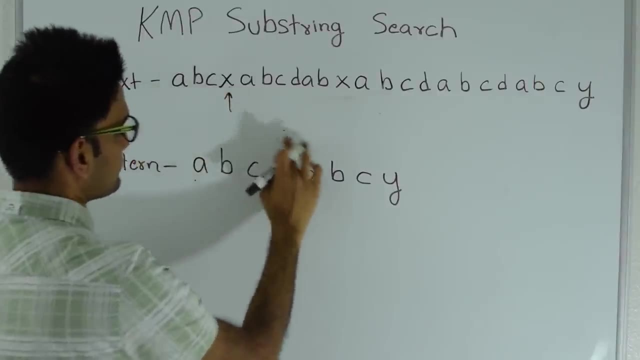 characters are unique, there is no way there can be a suffix, which is also a prefix. So what that means is our next comparison will start from XNA. Again, we'll understand it a little bit more in this example. So we compare A with X. 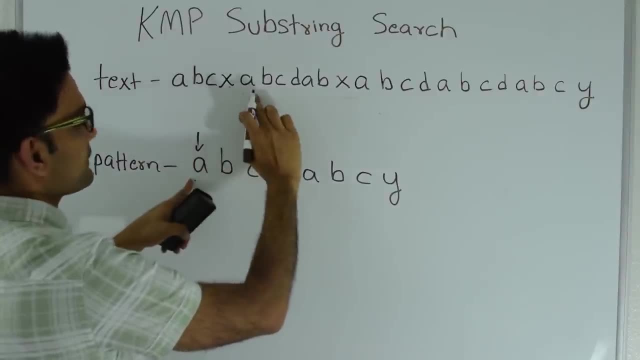 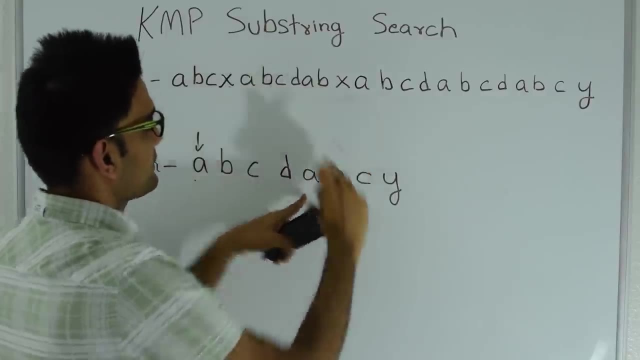 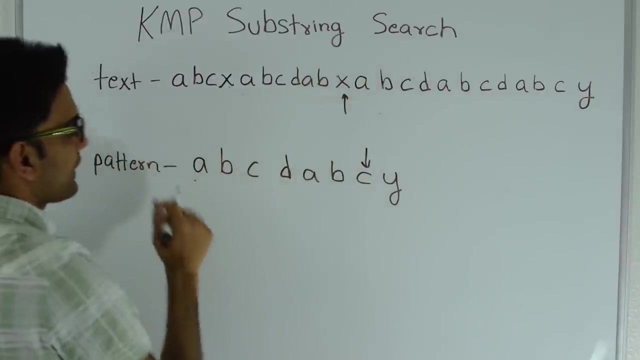 It's not a match. so we move to the next character: This A, this A is a match, this B and this B is a match. this C is a match, D is a match, A is a match, B is a match, X is not a match. So again, we check in this substring before C. 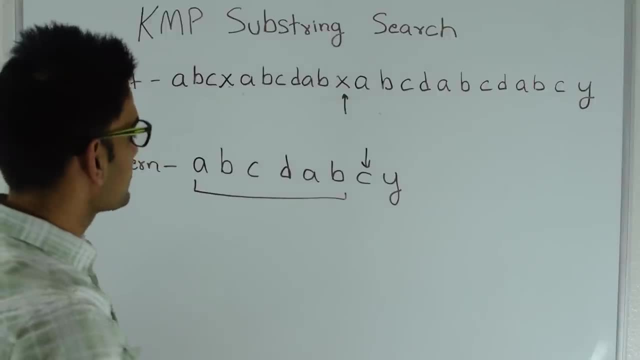 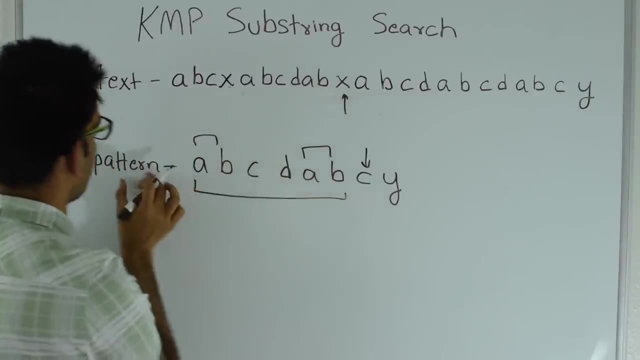 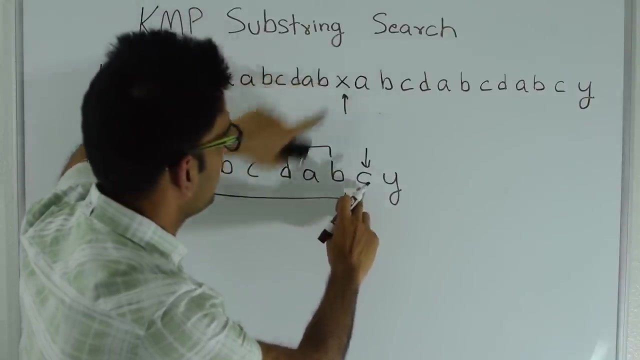 from A to B is there a suffix, which is also a prefix. So if you look here, this AB is both the suffix and the prefix of this pattern. What that means is, since we have matched till X till this point, the characters right before X must be AB. 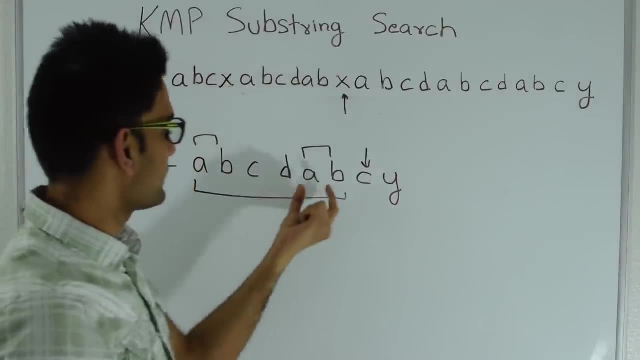 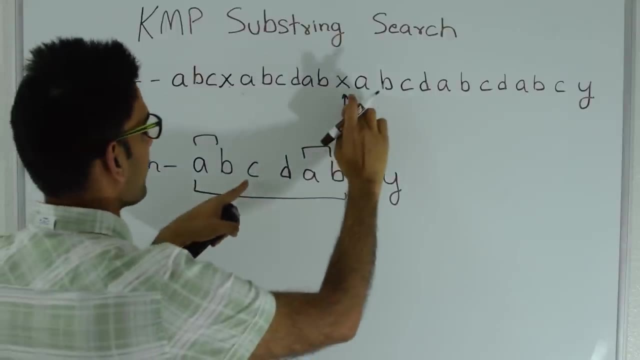 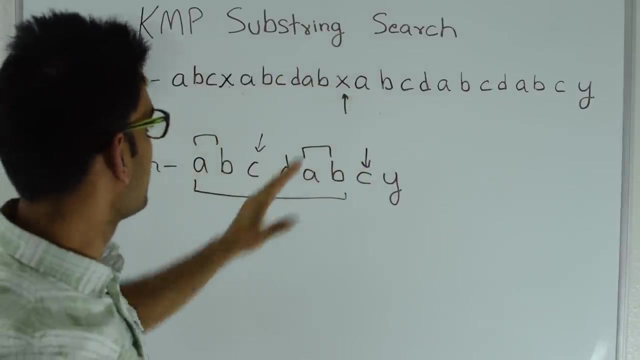 which is AB. So what that also means is that, since this is also a prefix, we don't have to match AB again, and the next match can start from X and C. So what happened here is we didn't have to look backwards in the string to see where to start then where. 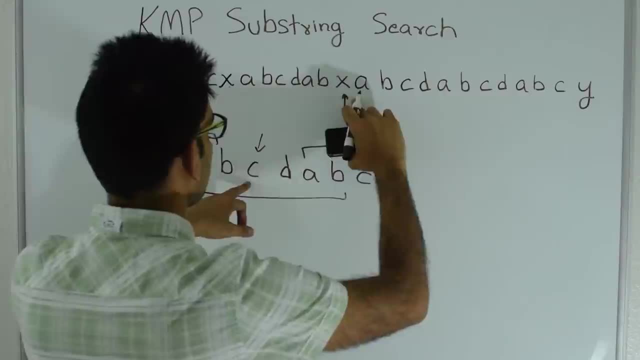 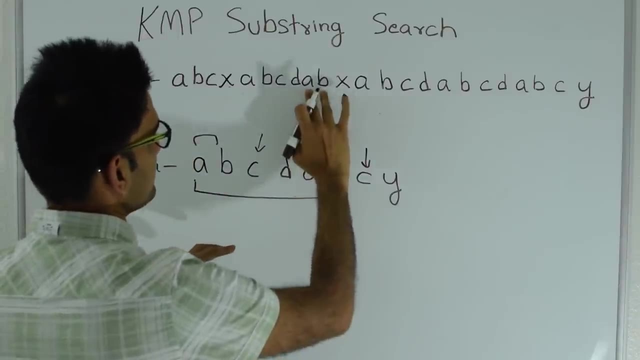 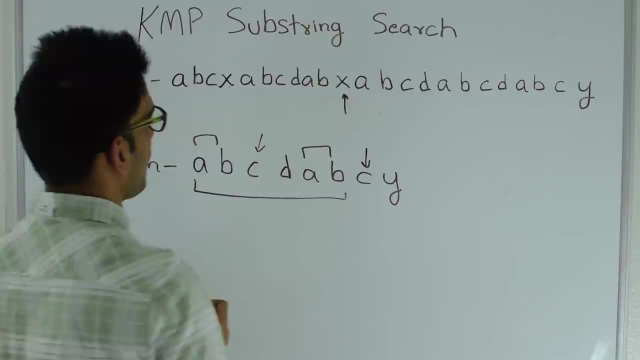 to start the next match from. We can start from right, here and here, since this suffix is this prefix, and since this suffix is this prefix, and since this AB exists here, we have already matched them, and so we start comparing C with X. So C and X is not same. so we check is. so we check is in. 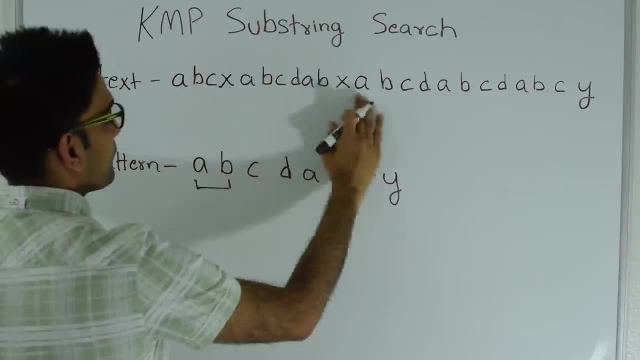 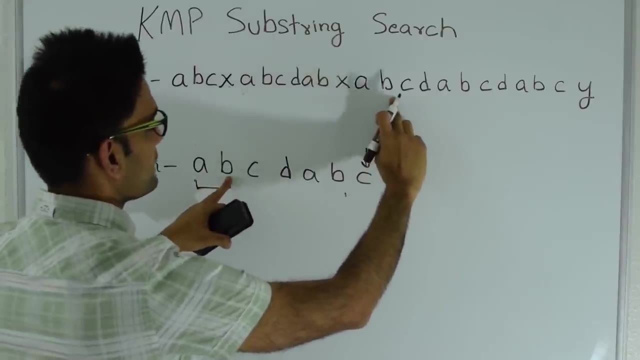 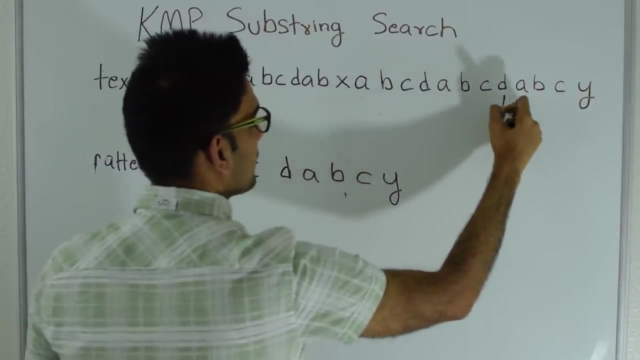 here is there a suffix, which is also a prefix. It's not. So finally, we start matching X with A. So X and A is not same. so we go to the next character: A and A is same, B is same, C is same, D is same, A is same, B is same, C is same. and then here we have a D and 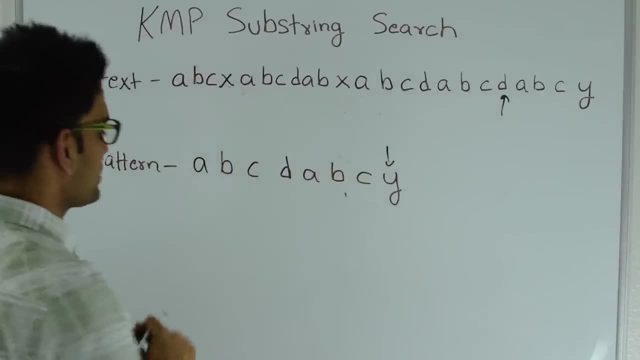 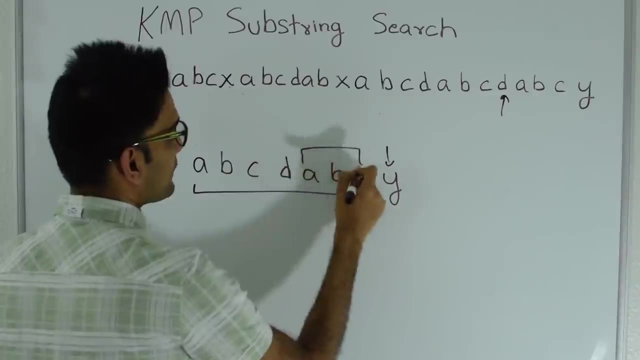 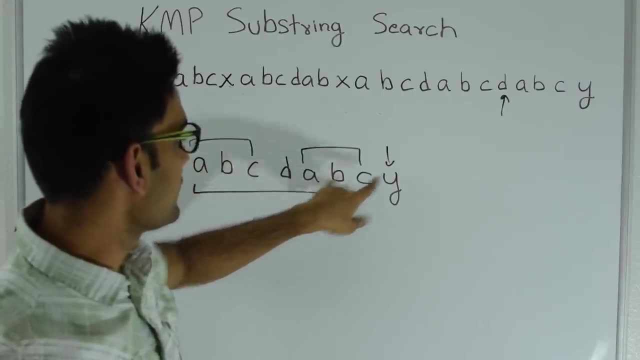 here we have Y, So again we check in this substring. before Y is there a suffix, which is also a prefix. So this suffix is also a prefix. What that means is, since we have matched till Y, this ABC must be right there. that's ABC. So what also means that, since this 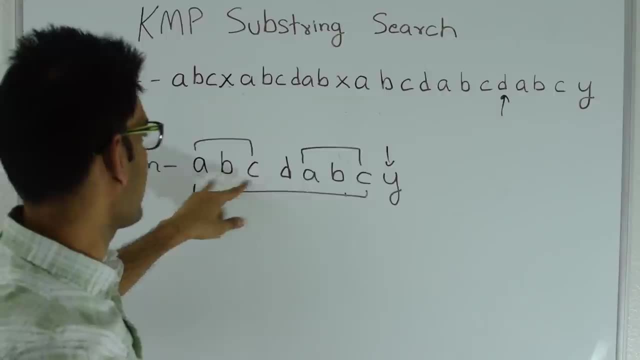 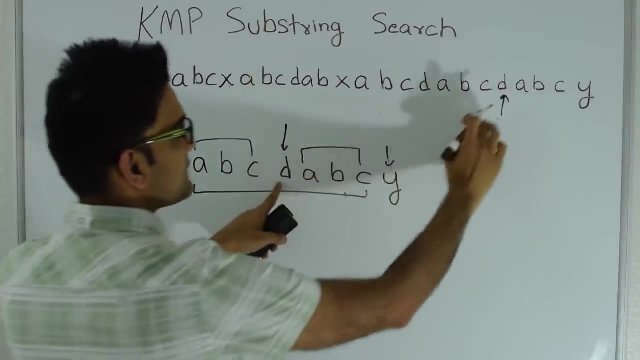 suffix is also a prefix. there is no reason to compare ABC again and the next check can start from right here. So this D has to be compared with this one. So this D and this D is same. then A is same, B is same, C is same and Y is same. So this: 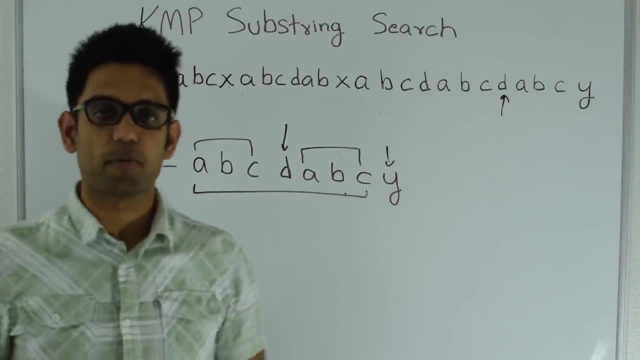 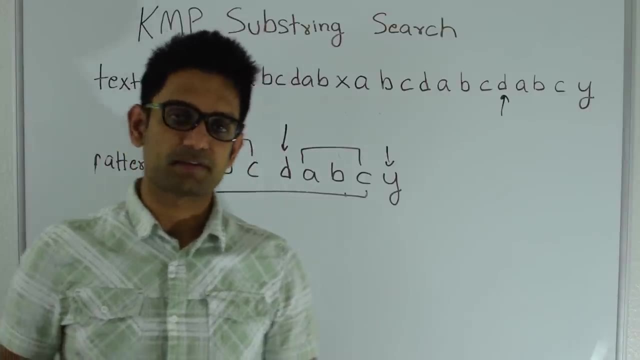 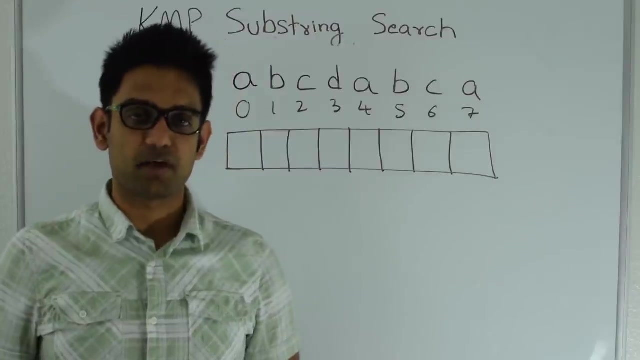 pattern exists in this text from this point onwards. Hopefully this helps you understand how the KMP search works using suffix and prefix information. So the only thing is: how do we do this efficiently? So the next section: let's look at that. So let's see how we'll efficiently compute if suffix is same as prefix and 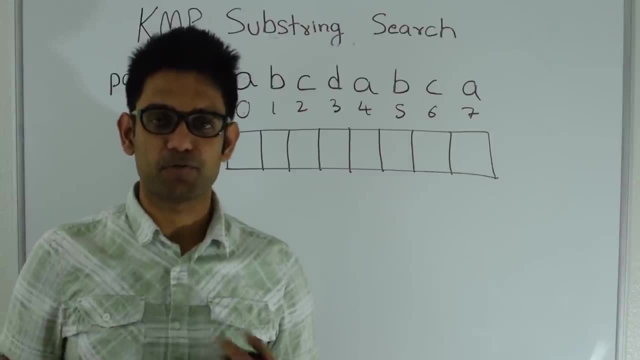 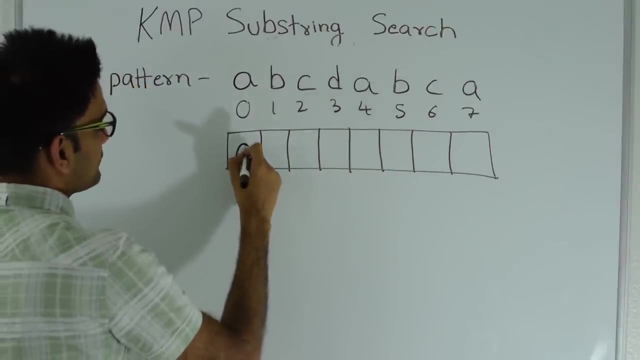 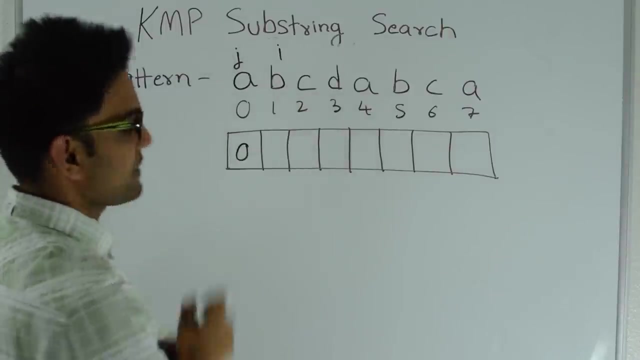 what point to start the check if there's a mismatch in the character between text and pattern. So here I have a pattern, ABCDABCA, So first is always zero. So this is my i and this is my j If there is a mismatch, if i is not same as j. 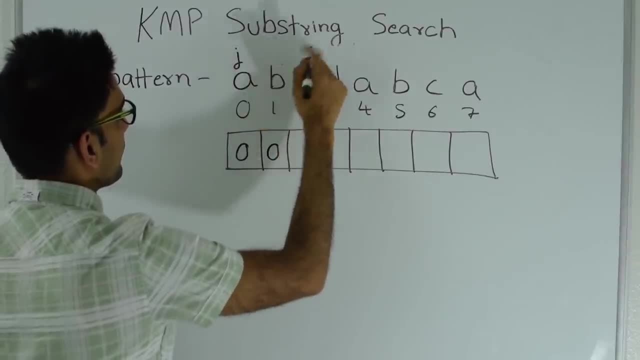 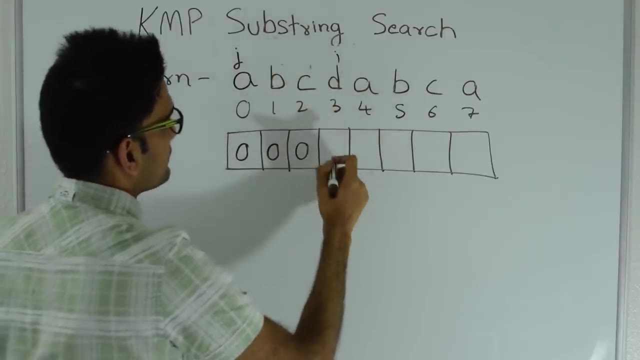 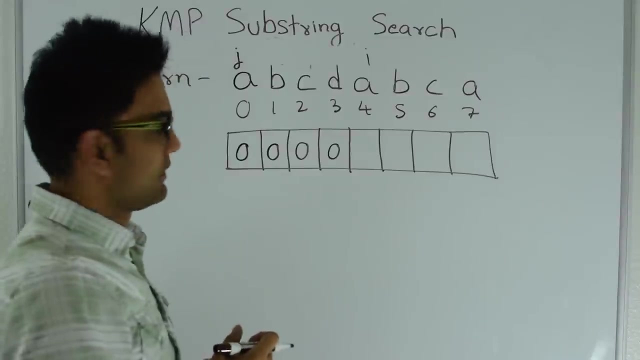 so we put 0 here and we increment our i Again. i is not same as j, so we put 0 here and we increment i. i is not same as j, so we put 0 here and increment i. Now i is same as j. So what we do is the value we put here is: whatever is the value of j. 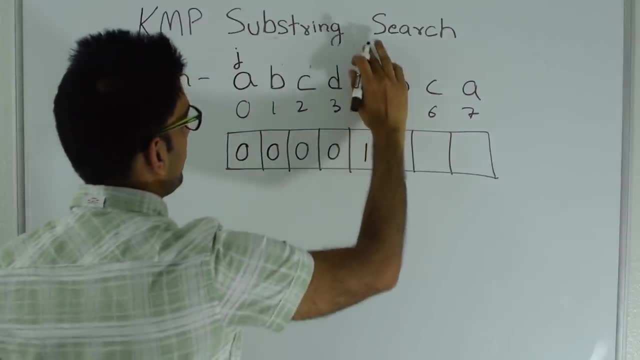 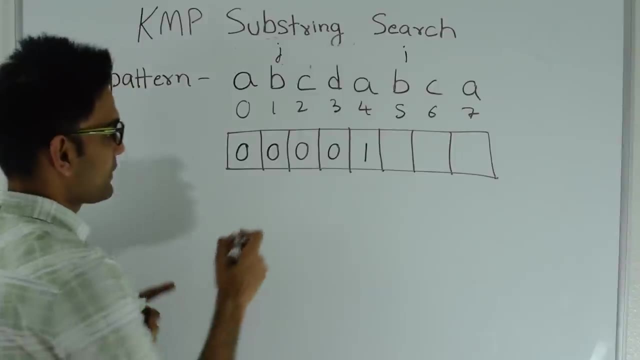 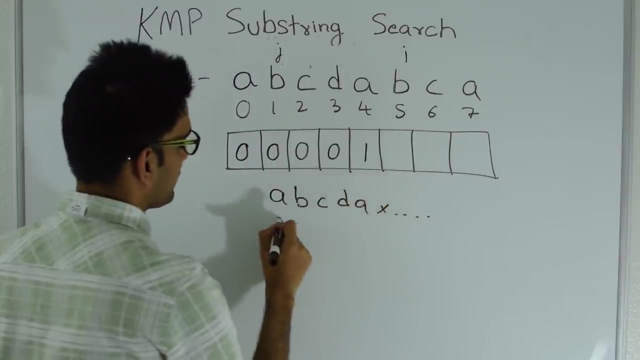 which is 0 plus 1. So this becomes 1, and then we increment both i and both j, So what this 1 means. So let's suppose our text was ABCDAX and so on and our pattern is ABCDAB. 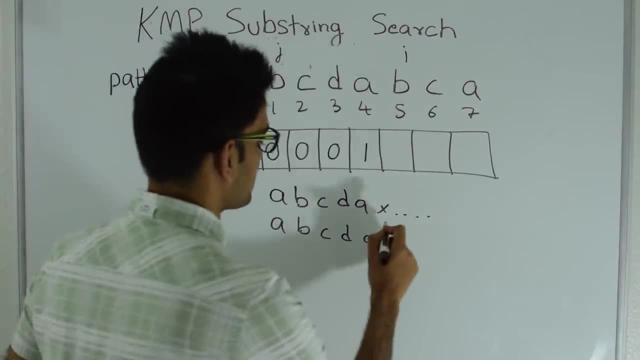 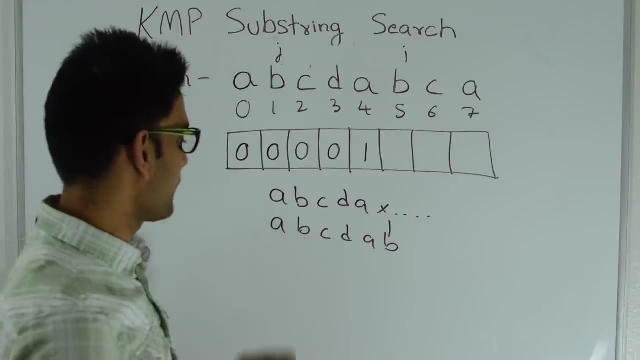 So there will be a match to this point, and this will be a mismatch right here between X and B. So point is: where do we start the next comparison in the pattern? So since the value here at the index of a is stored 1, it means that 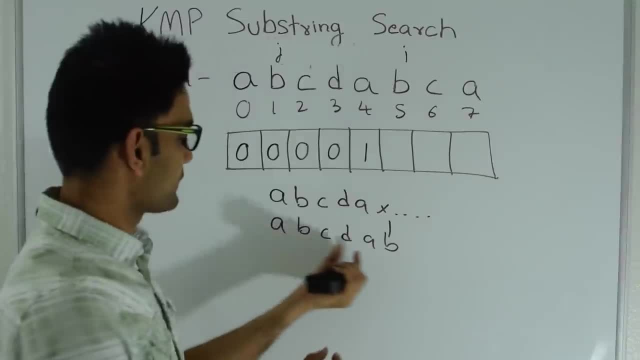 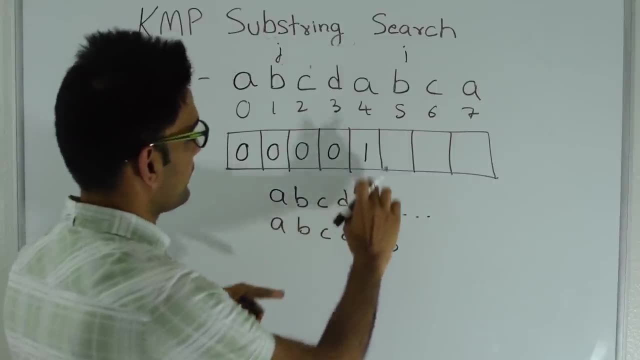 there is already. there is a prefix which is the same length as the suffix 1.. So we have already compared this a and this a. So the next point to check will be this X and this B. So this is where this 1 will come into the picture. 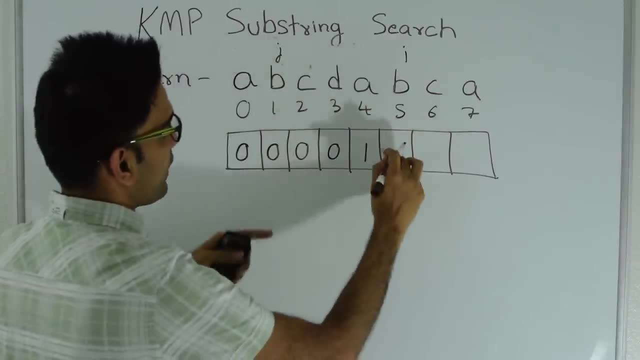 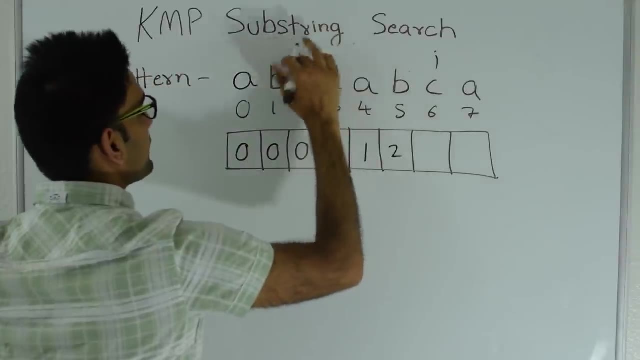 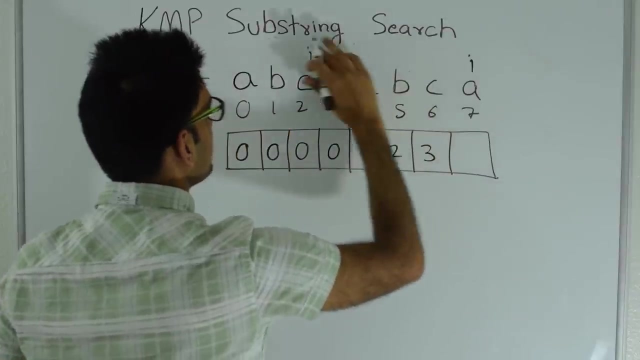 So again, B is same as B, So the value stored here will be the j, which is 1 plus 1, so that is 2.. And then we increment i and we increment j. C is same as C, So we store value 2 plus 1, 3, and then i goes here and j goes here. 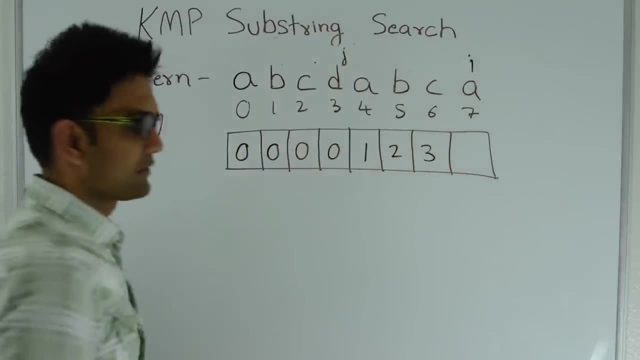 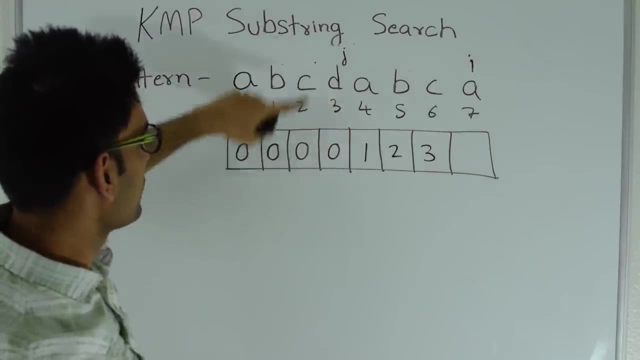 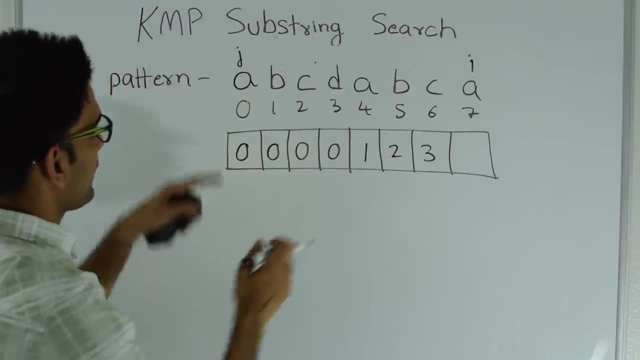 So now a is not a match with d, So this is little tricky. So what you do is you go to the value on the previous character, so that's 0. So j will become 0 and then you compare: is this guy same as this guy? So those, 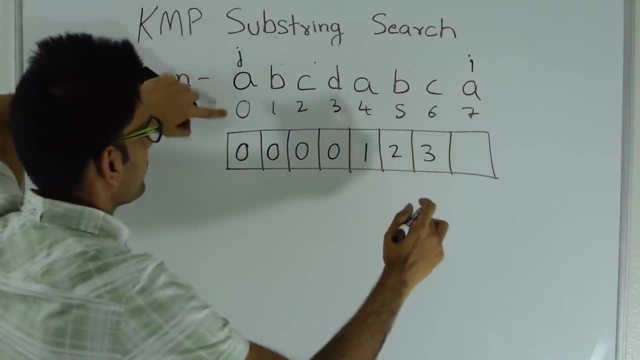 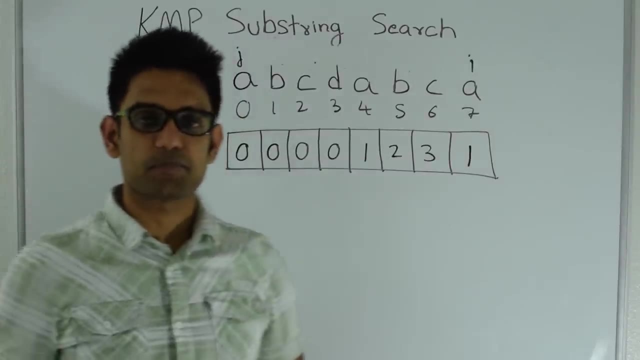 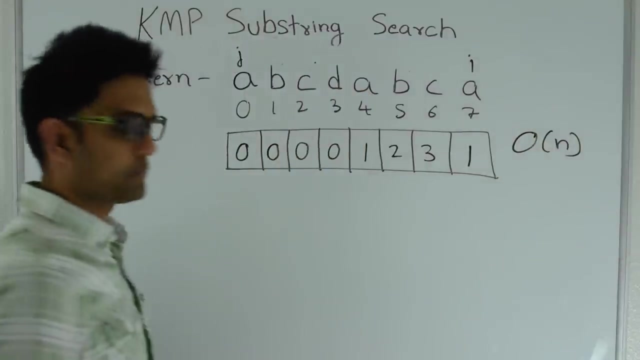 guys are same, So the value here will be whatever is the value at j, which is 0 plus 1.. So this is our temporary array and this array will help us doing the substring search efficiently. The time complexity to build this array is O and the space 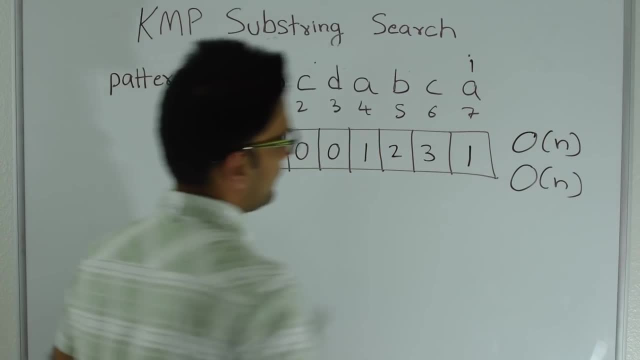 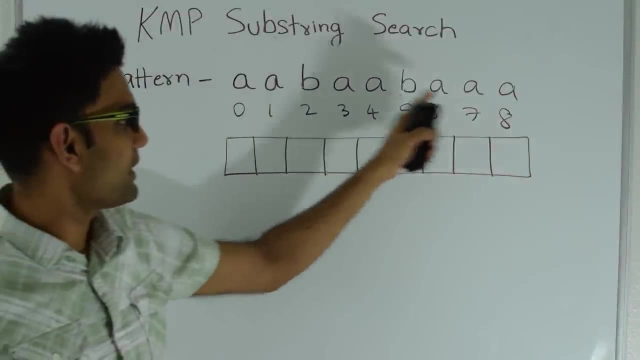 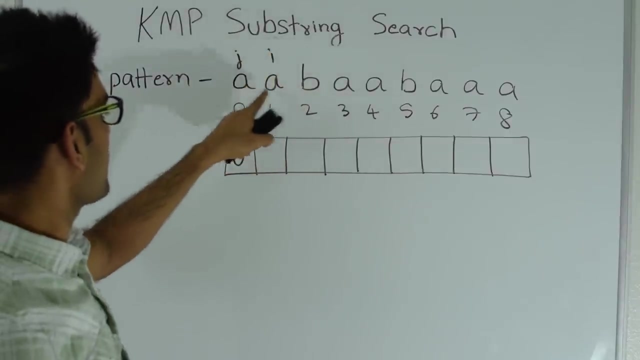 complexity is also O. Next, let's look at another example of how to build this array. So here I have a pattern, aabaabaaa. So first is always 0.. So i is herej is here. Since this i is same as j, the value here will be the value of j. 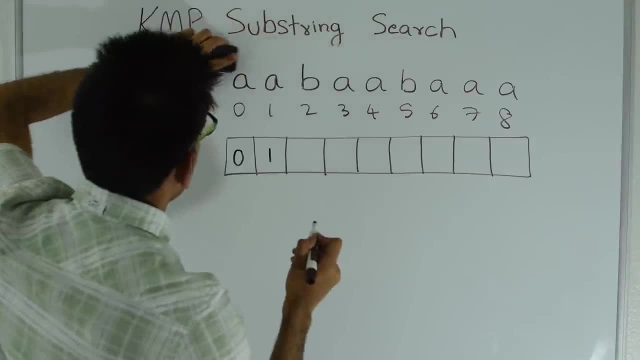 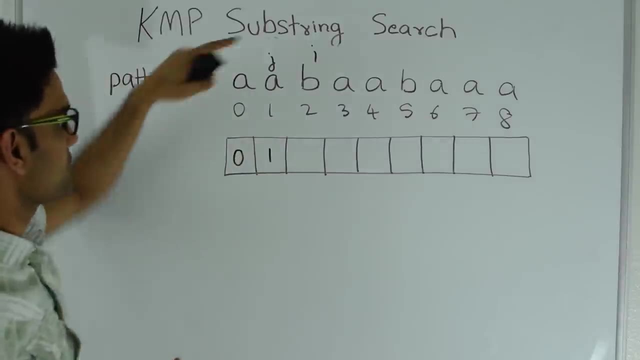 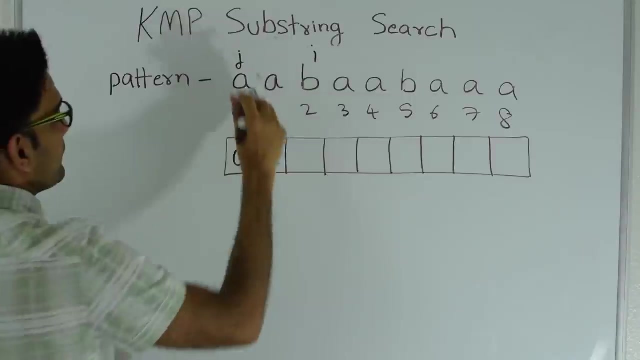 plus 1.. So this is 1, and then increment both i and j, So i comes herej comes here. This value is not same as this value, so the next point of j will be the value in the previous character, which is 0.. So j becomes 0. This is not same as this, so 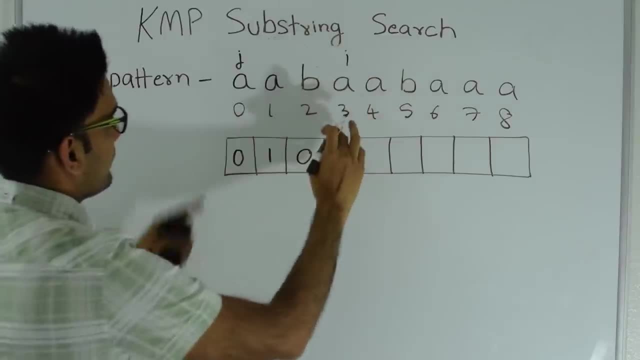 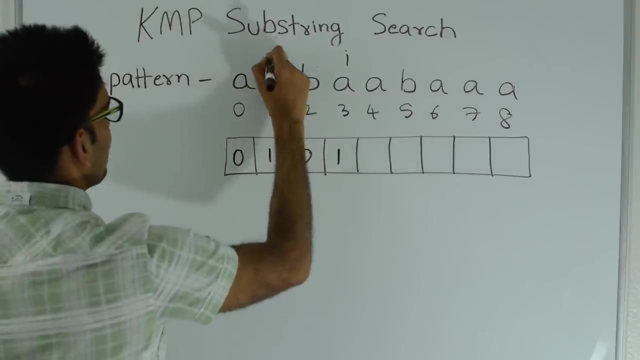 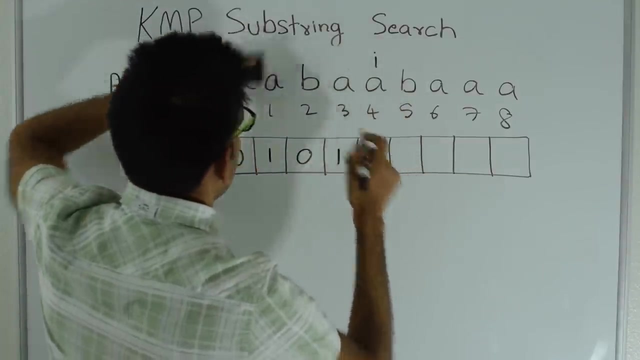 this value becomes 0 and we increment i. This is same as this, So the value here will be j plus 1.. So this is 1, and then we increment both i and j Again. this is same as this. So this becomes 2 and we. 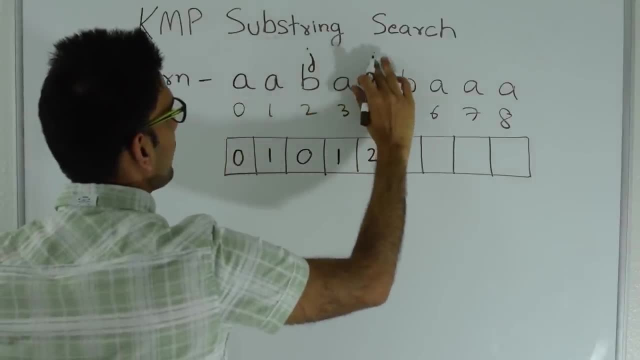 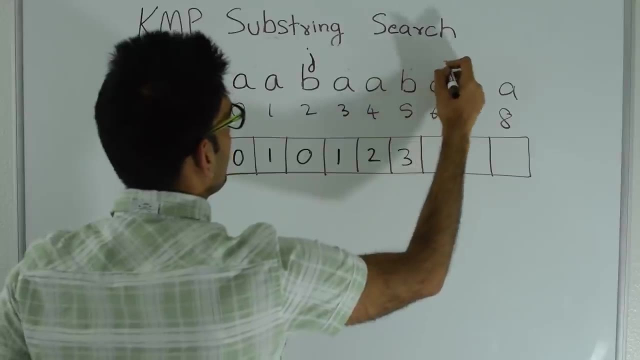 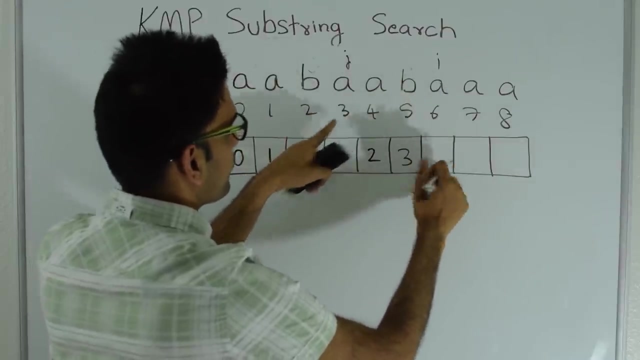 increment both i with both j and i. Again, this is same as this. So the value here will be 2 plus 1 is 3, and we increment both i and j- Again, they are same. so value here will be 3 plus 1 is 4, and we increment i and then j. 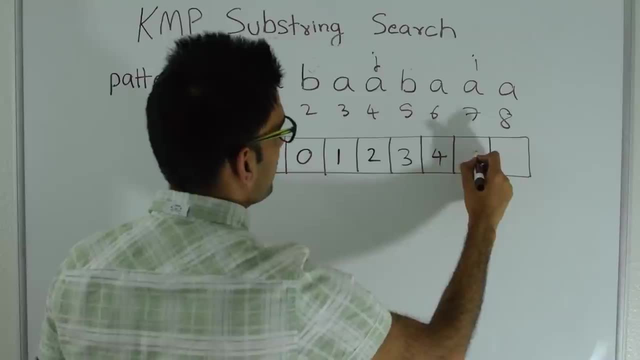 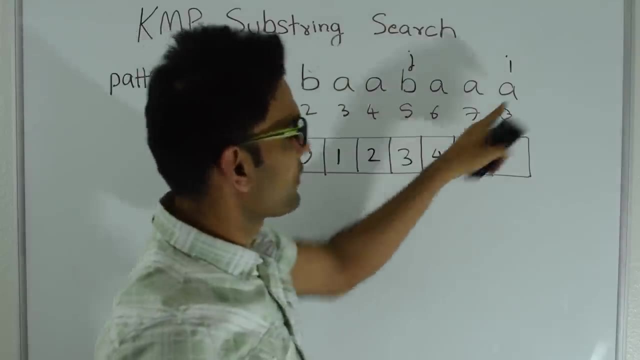 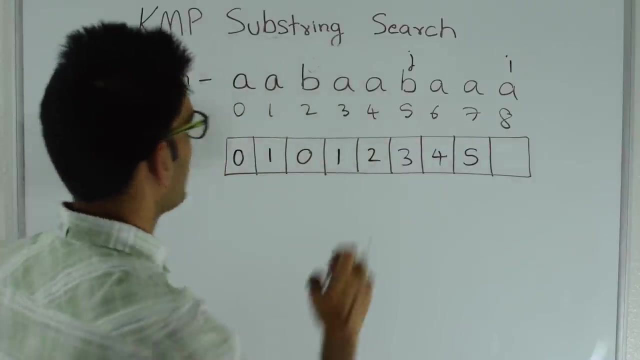 Again, they are same. so value here will be 5 and we increment i and then j. At this point b is not same as a. So the next point j will be is the value in the previous character, which is 2.. So j jumps directly to 2.. Again, this a is not same. 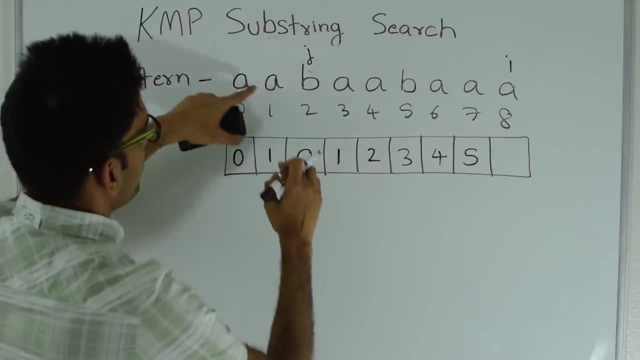 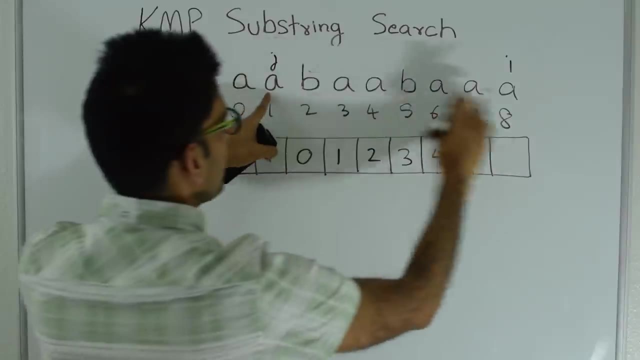 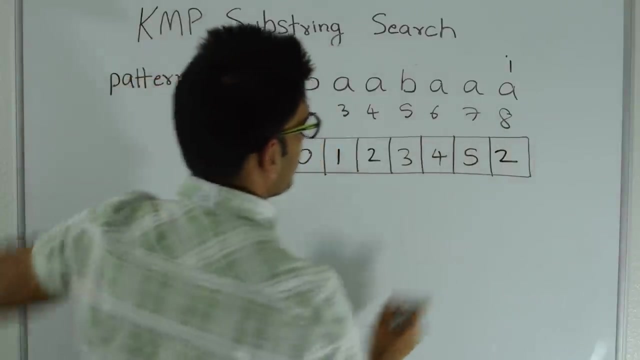 as this a. So j will jump to the value in here. So that's 1.. So j comes to this point. At this point, this a is same as this a, So the value stored here will be whatever j is. So 1 plus 1.. So this is 2.. So this is how we build a temporary array for 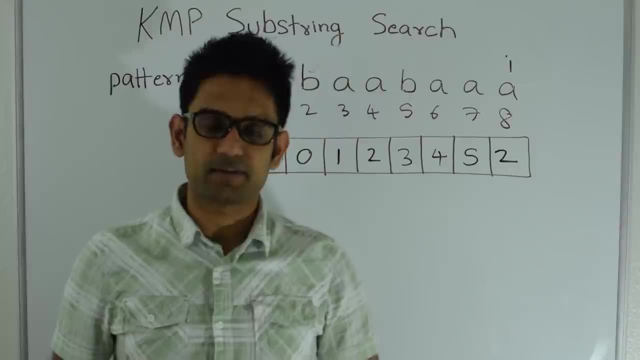 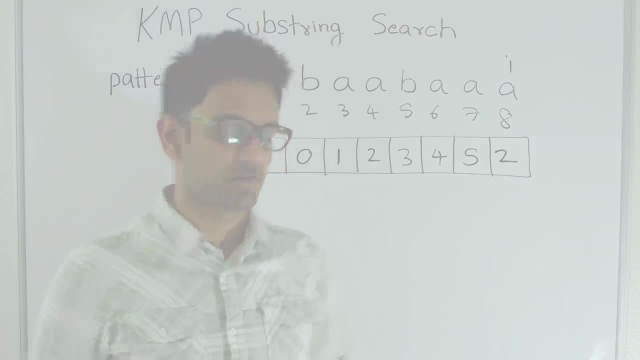 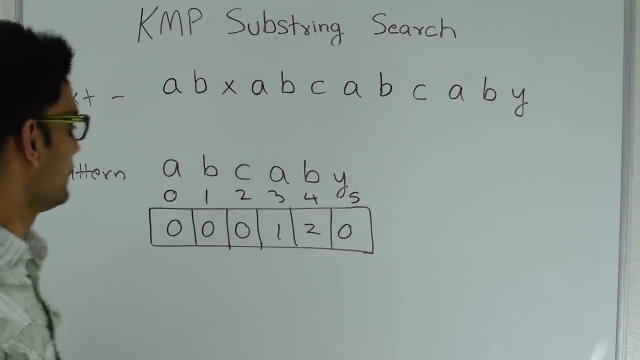 this pattern. So again, the time complexity is O and the space complexity is also O. In the next section let's use this array to actually do the substring search. Finally, let's apply the substring search on this text for this pattern. So I've pre-built my array using using the 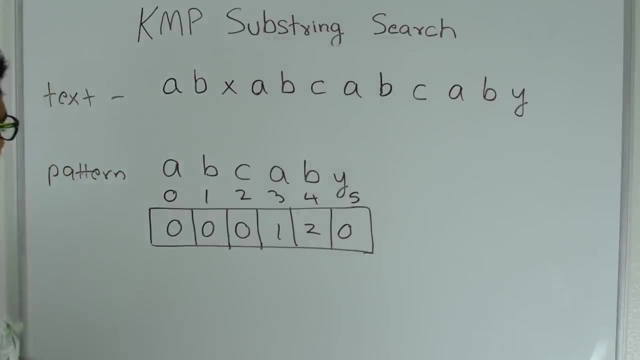 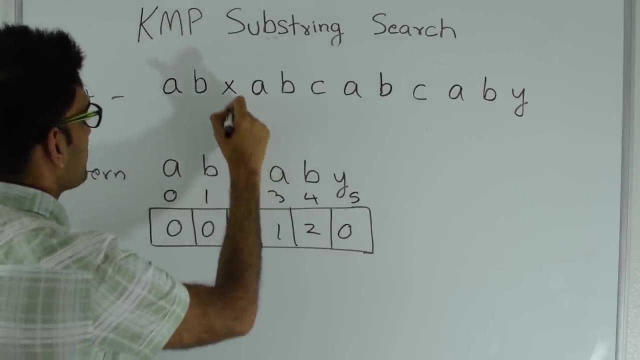 logic which we discussed in the previous section of this video. So now we compare a with a, So they are, they're same. then b is same, So this c is not same as this x. So then what is the next point? So, since we're not going to look, 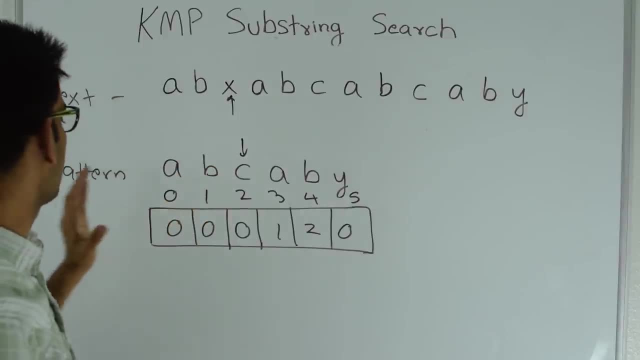 back in the of text. we check what is the next point. we compare this pattern and this text. So the value at. we go back to b and check the value. The value here is 0. So the next point of comparison will be this a and this x. because index, because we 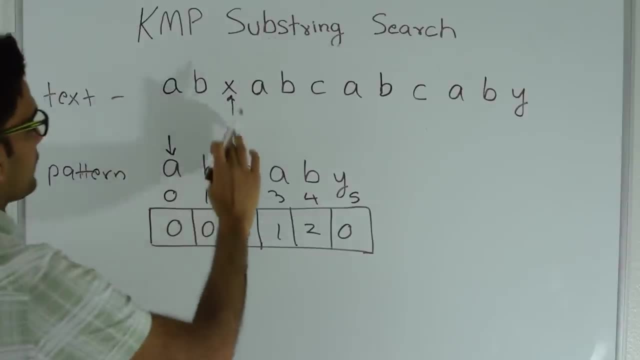 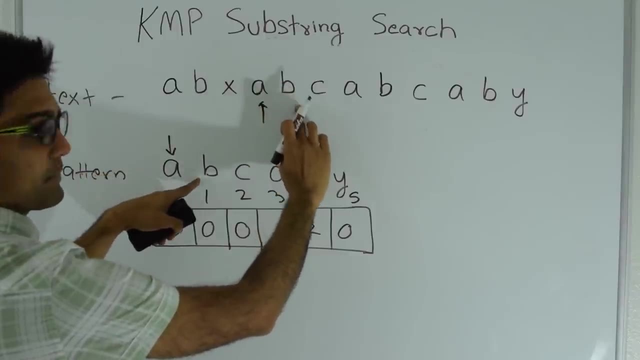 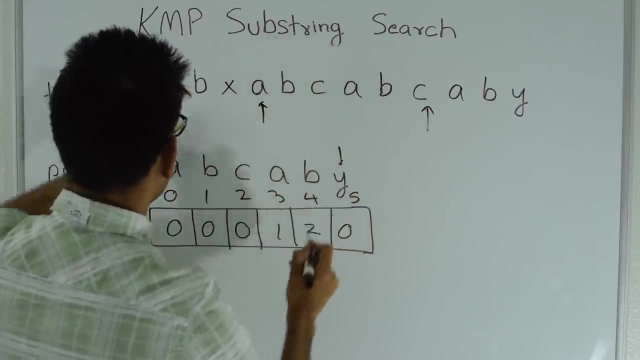 start looking from index 0, which is a. So this a is not same as this x, so we move forward. This a is same as this a, then this b is same as b, c is same as c. Again, a is a match, b is a match, and then at this point it's not a match. So 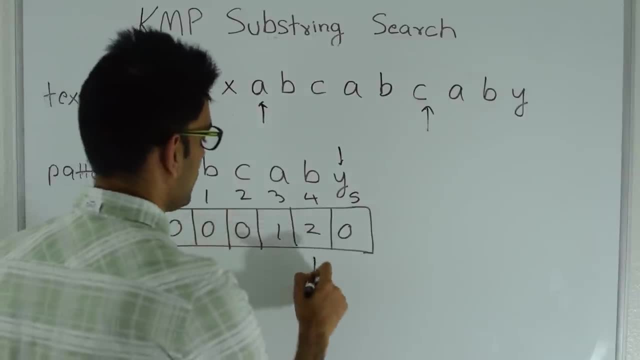 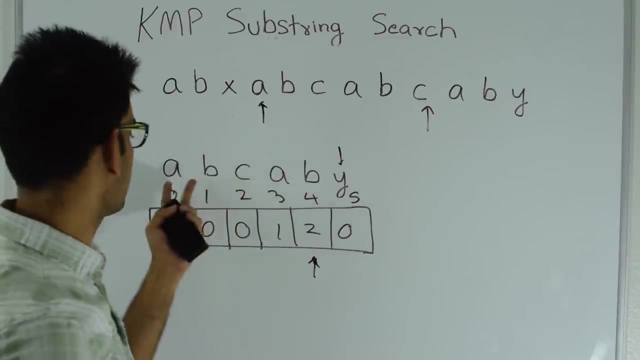 again. we go back here and then 2.. So what this 2 is saying is that there is a prefix of length 2, which is also a suffix, which is clear. This ab is a this, this ab and this ab are prefix and suffix. So what that also means is that there